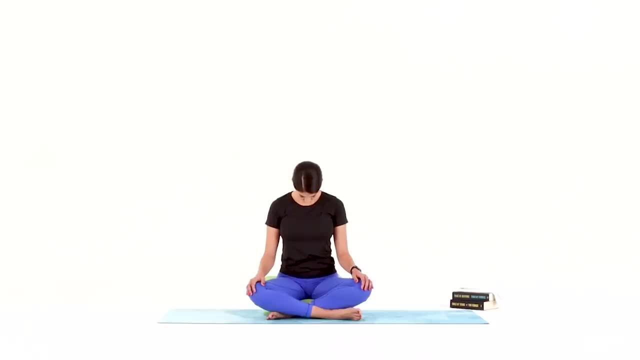 So notice how it feels for you today And if it feels good, try rocking your head side to side, gently and slowly. yoga is not a game of freeze tag. you are more than welcome to fidget or move or find something that feels even better for you. trust that your body will tell you if you've ever gone too far. 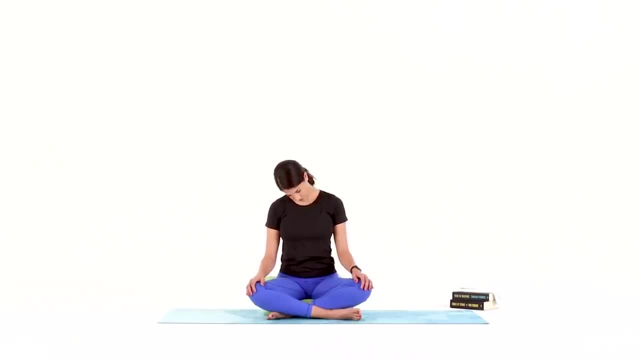 through pain or strain, and we never push through pain or strain. now, with your hands on your knees, palms down, pull your chest forward and lift your chin up as you roll your shoulders back and take a big inhale, then exhale to round your spine, tuck your chin. 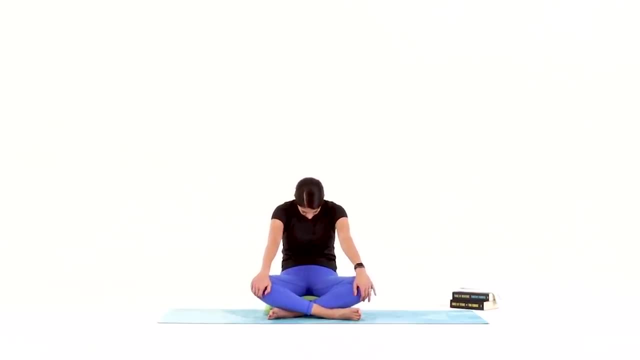 cave your chest and press the space between your shoulder blades back, warming up the spine synovial fluid along your spine. let's do that again. pull your chest forward, lift your chin up, roll your shoulders back, even lift your chest up, then tuck your chin round your spine, cave your chest and press back just one more time. pull. 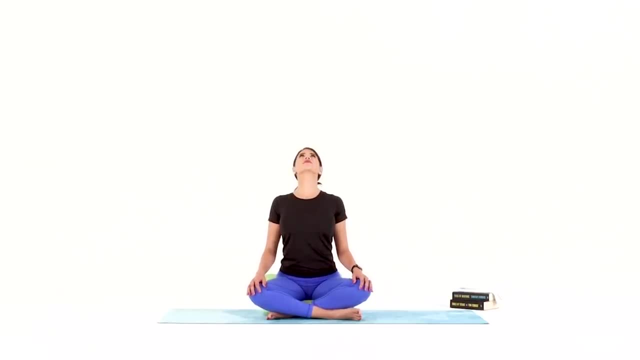 your chest forward, lift your chin up, roll your shoulders back. then tuck your chin round your spine, cave your chest, press it back and come back to sitting tall with a neutral spine and notice any new sensation. then open your eyes, if they weren't open already, and lower your arms down by your side, so your 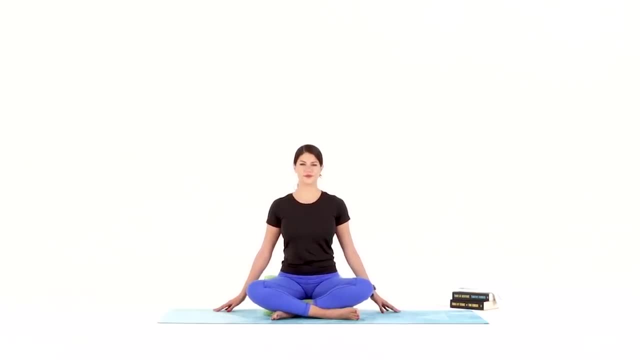 fingertips might touch the ground or your prop, or they just hang out by your sides and reach your left arm up towards the ceiling. stretch your arms up and down and lift your chin up and lift your chest up. stretch up through your fingertips and right here you might feel a decent 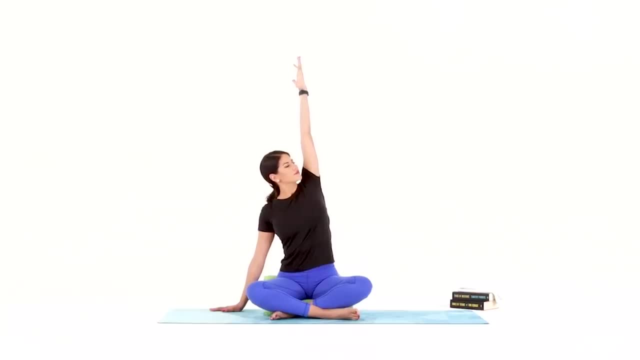 opening through your chest and your shoulder. you're more than welcome to just stay here and breathe, but if you want to take a little bit further, then lean into your right side. arc your left arm over. you're not caving your chest forward or letting your head hang forward. keep your chest tall, just. 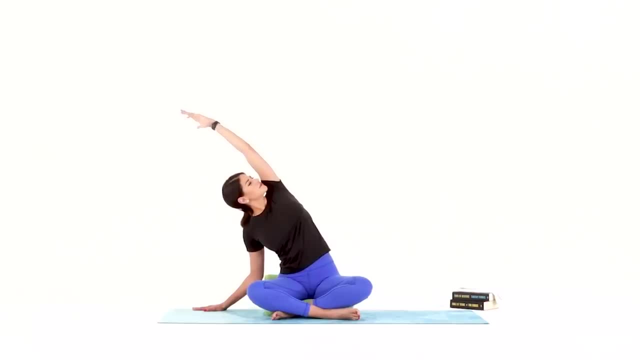 lengthen your body from your left hip bone through your left fingertips and use your breath to create space between your left ribs for three minutes. 3., 2., 1. back to center. lower your left arm down. take a moment here to reset. notice the. 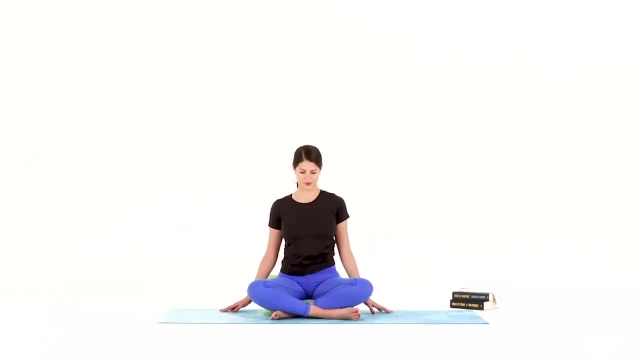 blood flow down your left arm and then we'll switch sides. reach your right arm up to the ceiling, notice any stretch that you might feel in your chest or shoulder, and if you did on the other side, then arc over leaning into your left side. keep your chest open so you're not caving in, and then take a deep breath for 5 minutes. 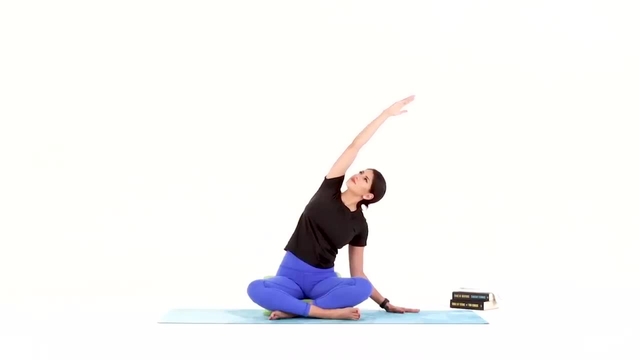 forward. lengthen from your right hip through your right fingertips and use your breath to create space between your right ribs. for three, two, one. come back to center. lower your right arm down and notice the blood flow down your right arm. then, for a twist, place your left hand on your right knee. 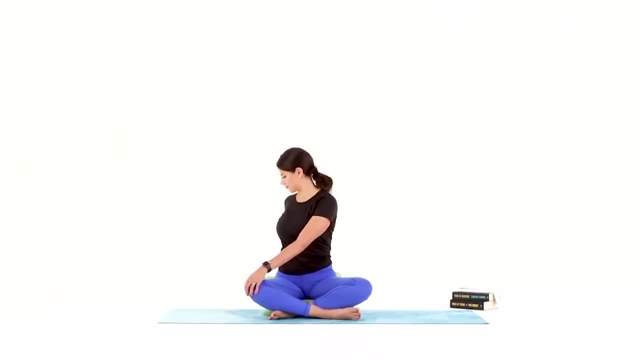 and place your right hand wherever it lands behind you, twist your upper body to the right, through your chest, shoulders, even through your chin and your eyes. then, once you're in your twist, you're there. no need to yank yourself further, just hold and breathe in and out through your nose. 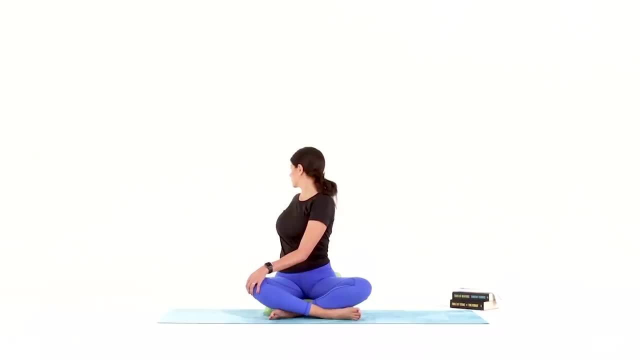 three, two, one. come back to center. pause for a moment, notice how you feel. then twist to your left. place your right hand to your left knee. left hand plants behind you wherever it lands. then twist your upper body to the left through your chest, shoulders, chin and eyes and notice how your breath feels within this twist. 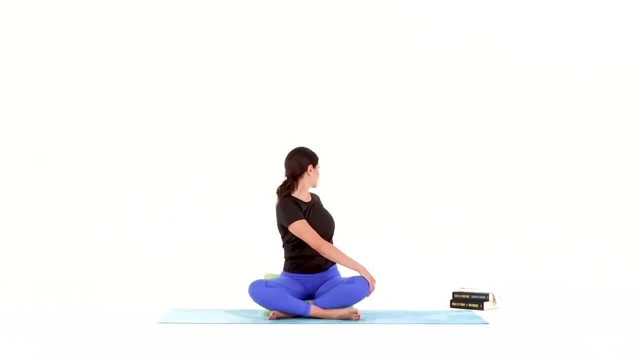 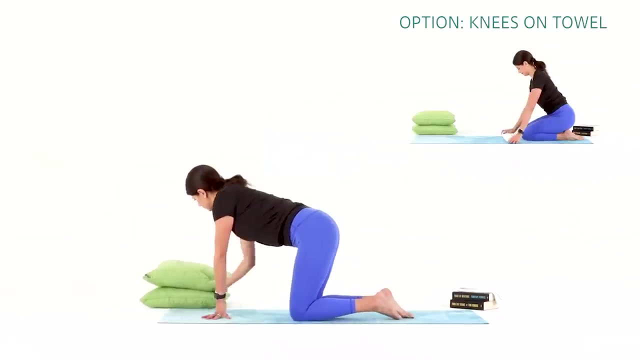 three, two, one. come back to center and pause. notice any new sensation. then make your way into a tabletop facing the front of your mat on your hands and knees. i do recommend placing a hand towel underneath your knees for extra cushion. you want your right hand to be at the same height as your left knee and your right hand to be at the 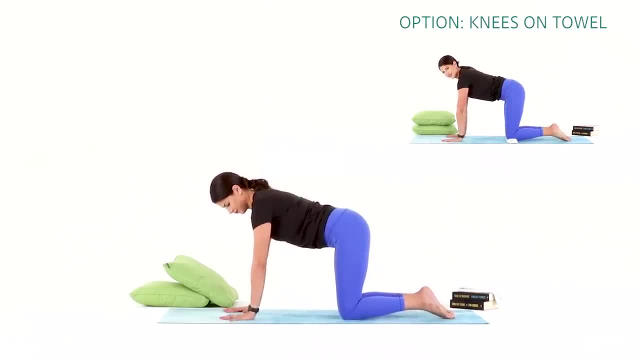 knees directly underneath your hips so that your thighs are parallel with each other, and your hands directly underneath your shoulders, so that your arms are parallel with each other and to create the top of your table. you want your back flat, so instead of letting your belly drop down towards 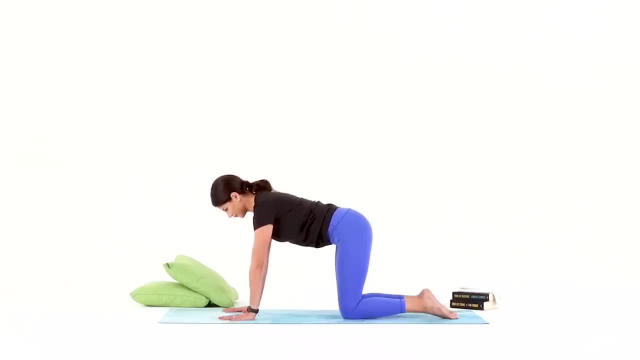 your mat. use your core to pull your navel in towards your spine, and that will hold your core in place and flatten out your back. bring your neck up in line with your spine so that the back of your head and your back are all the table top. this is an active pose, so if you were to hold it, 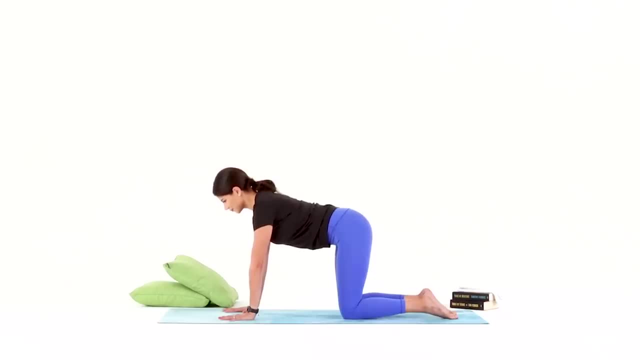 for even a minute with this core engagement, you would feel your core working. this is your neutral position in tabletop. so to add on cat cow spinal waves, which are very common in our yoga practice, first for cow pose, drop your belly down towards your mat and lift your chin up. this is stretching the whole front. 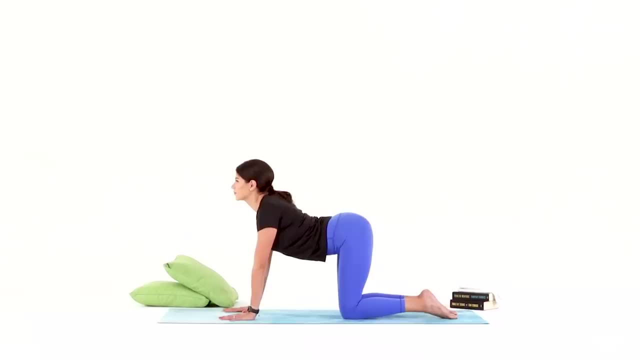 line of your body should feel good, and typically we match this with an inhale, so breathe in, then exhale. come back to your neutral position in tabletop. pull your belly in neck is in line with your spine for a cat back round your spine, tuck your chin, even tuck your. 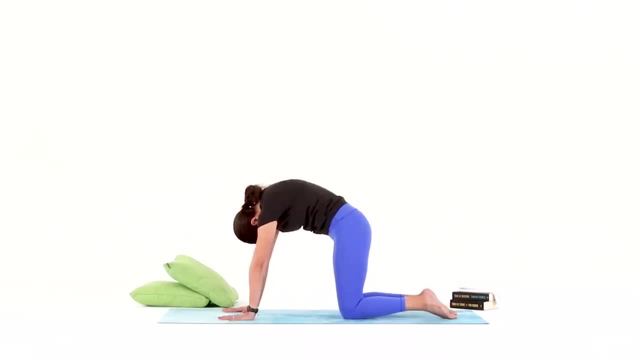 tailbone like a scaredy cat. you're pressing everything away from you and you're going to be able to pull your navel in towards the mat and then pull your navel in here, take a breath in through your nose, big breath out, and come back to your neutral position in tabletop. 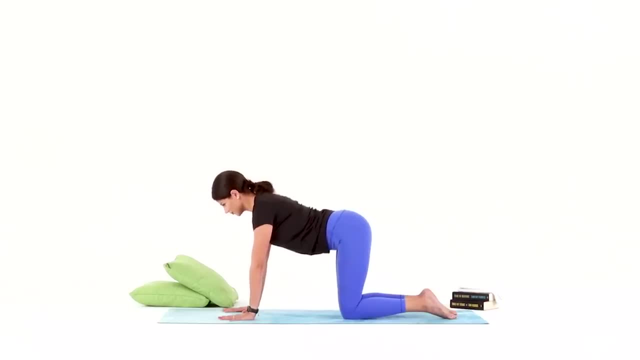 and again for cow pose. drop your belly, lift your chin, feel the stretch along your front. inhale, exhale. come back to tabletop neutral. spine belly pulls in for a cat back round your spine. tuck your chin, tuck your tailbone, pull your navel in. 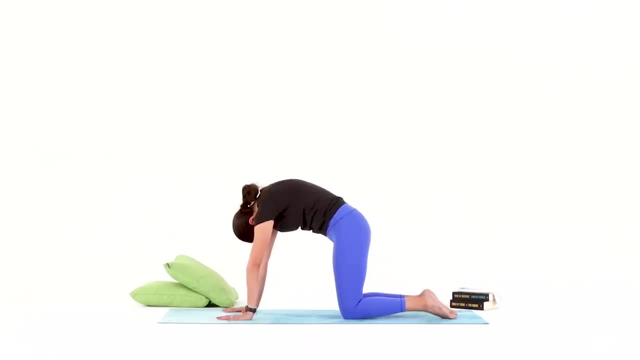 even here for one full inhale and exhale and come back to your tabletop. one more of each for cow pose. drop your belly, lift your chin, big breath in big stretch. then exhale back to tabletop. nice for cat back round your spine, tuck your chin, tuck your tailbone. navel pulls in big breath in big. 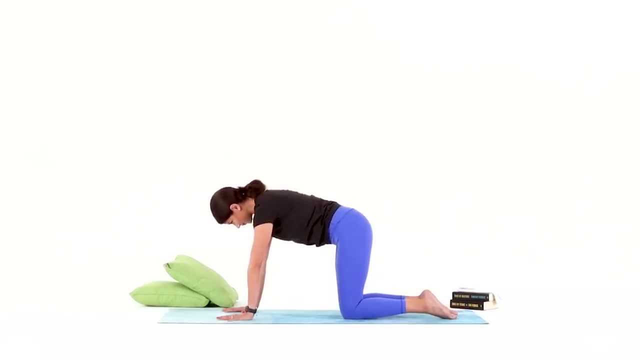 breath out and come back to tabletop. well done. meet me in child's pose. separate your knees wide towards the edges of your mat, bring your big toes to touch behind you, and it's okay if they don't touch. I just want your shins in the shape of a triangle and you're going to do a cat back pull. 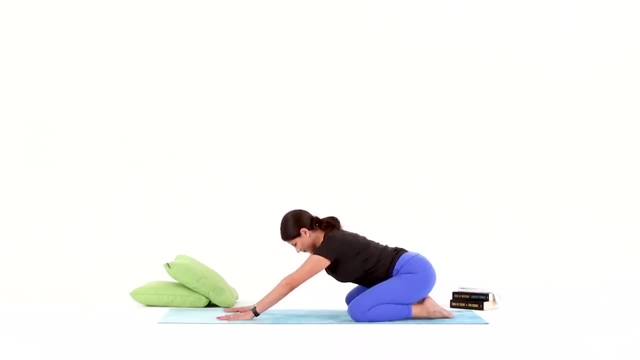 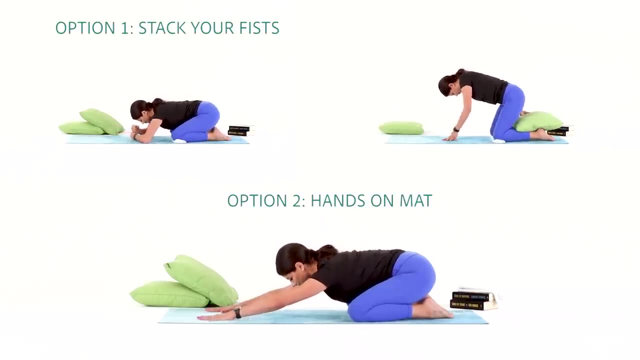 and sit your hips back towards your heels- and you can always place a pillow underneath your hips for more support- and lower your chest down towards your mat and extend your arms out long in front of you. rest your forehead on your mat, but sometimes this is a little too intense to 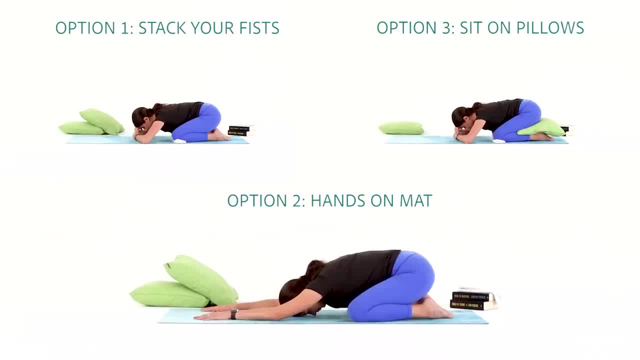 start so you can always stack your wrists or your fists underneath your forehead in all. the word yoga in the pg faceы- the word yoga in the pg face is the term that sunday morning is usually in the pg face. the symbol is the canal. Tú means to unite, and what you unite is your mind and body. so from the yogi in 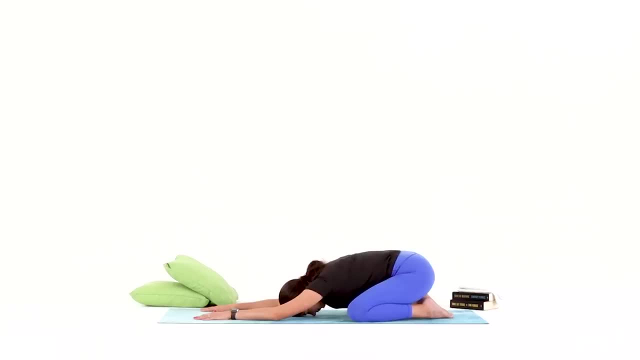 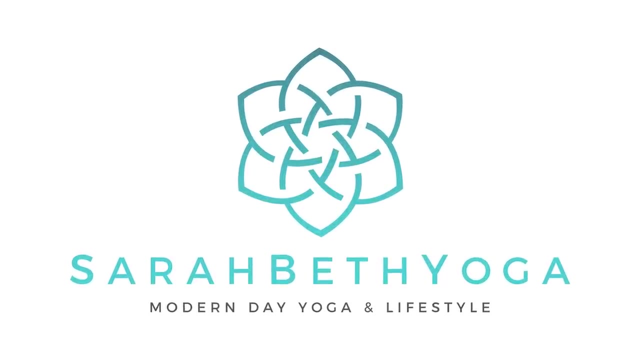 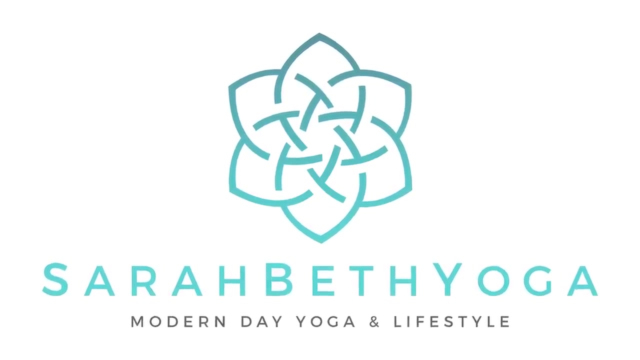 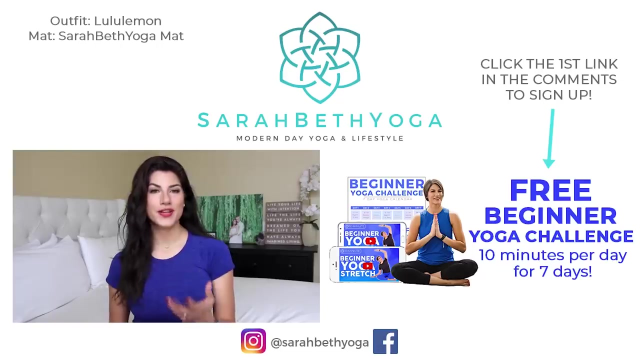 me to the yogi in you. namaste you well done. hi. i'm sarah beth and i'm here to help you get fit, happy and healthy through yoga. i created this beginner level yoga video as an easy and fast way to wake up your body and increase.